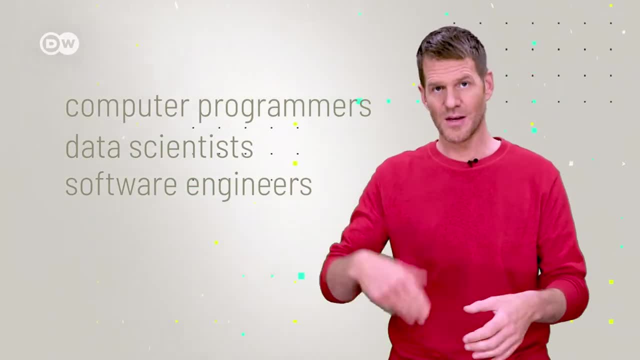 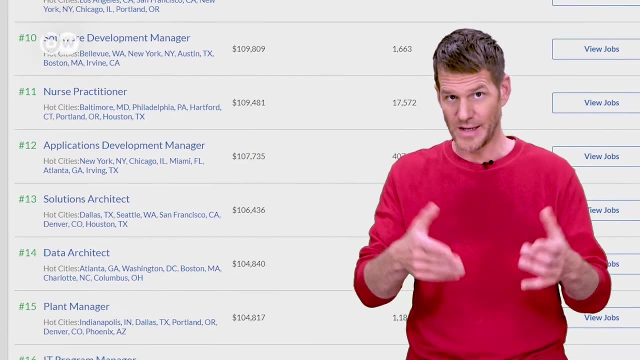 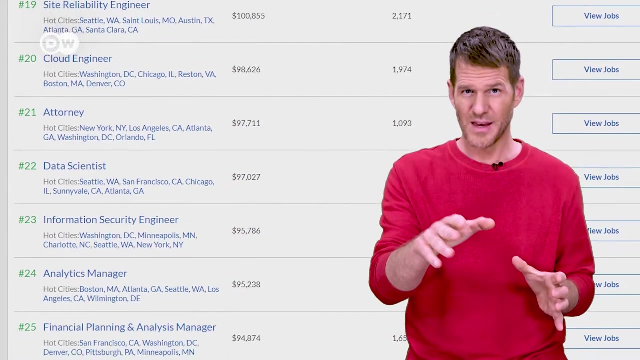 I'm talking computer programmers, data scientists, software engineers and so on. They rank among the highest paying jobs. Still, the number of vacant positions is quite large. The reason: There are not enough graduates with the required skill set. So, thinking of your kids, there are loads of job opportunities coming up. But 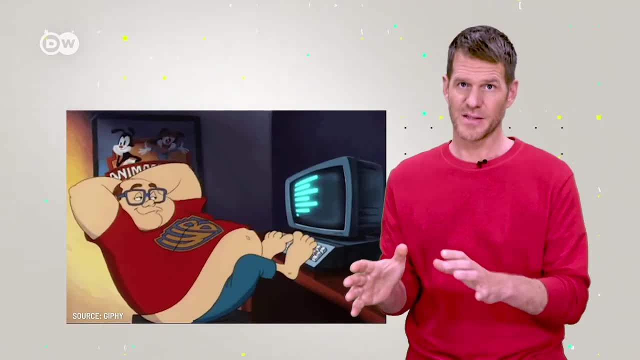 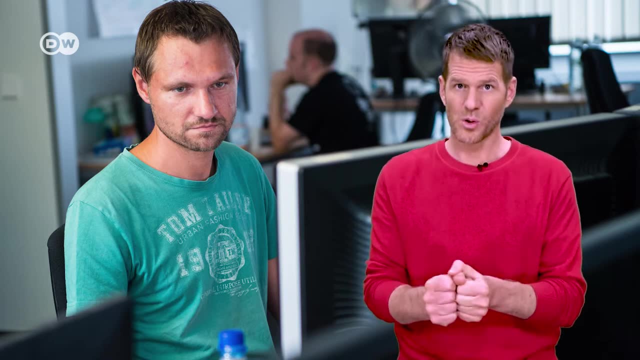 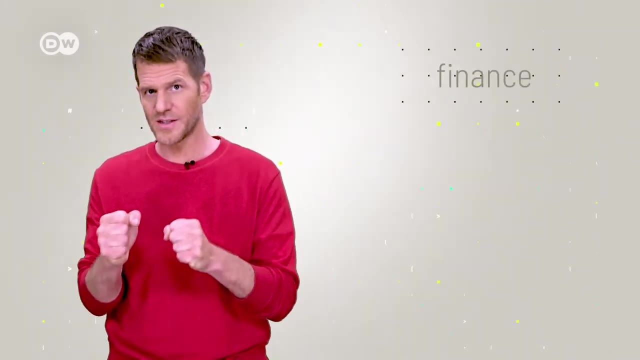 even if your kid doesn't want to work in tech, a basic understanding of coding will be important in every field. Already today, thousands of industries depend on computer programs to run their operations, And it's not just data analysis. Code is the backbone of work in the finance. 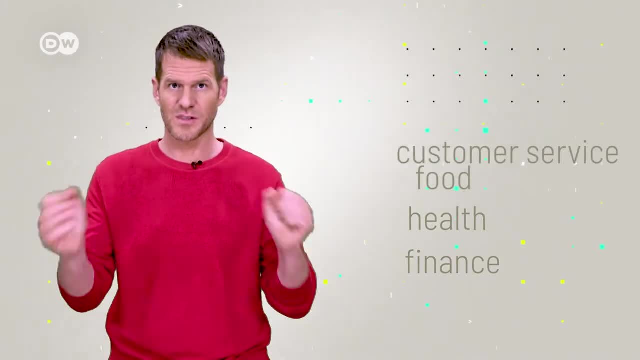 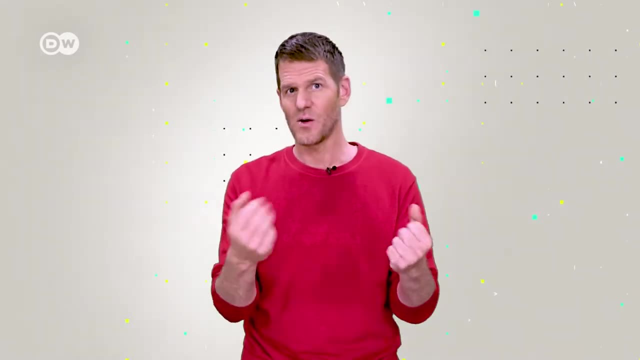 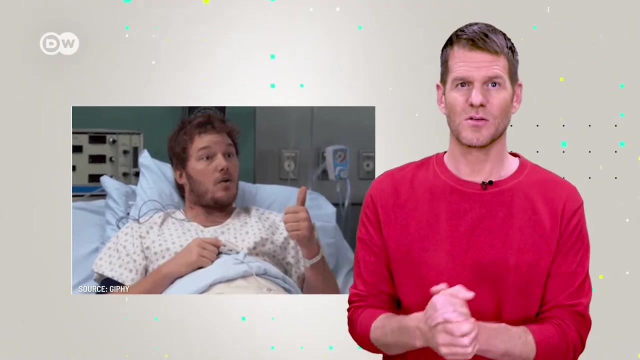 sector, the health sector, the food industry, customer services or education. So even if your child wants to be a doctor, it's important that it understands how exactly artificial artificial intelligence works, for example, Because it might help in analyzing data sets. 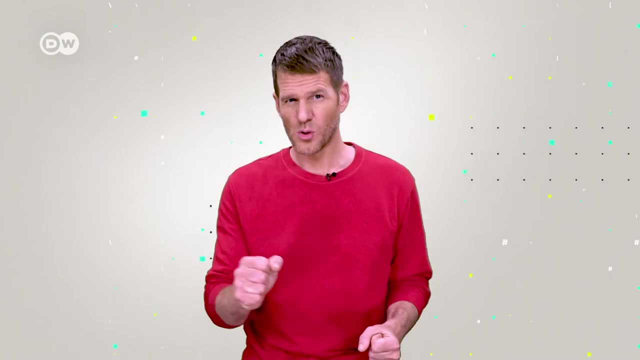 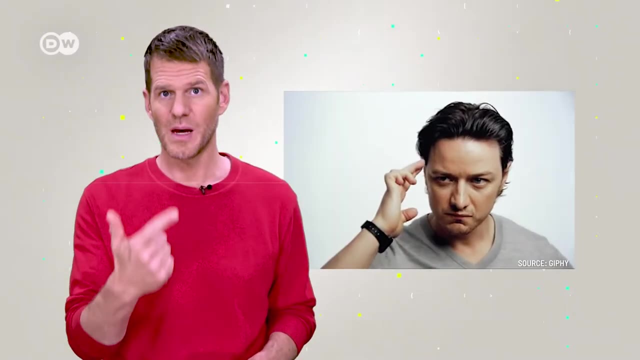 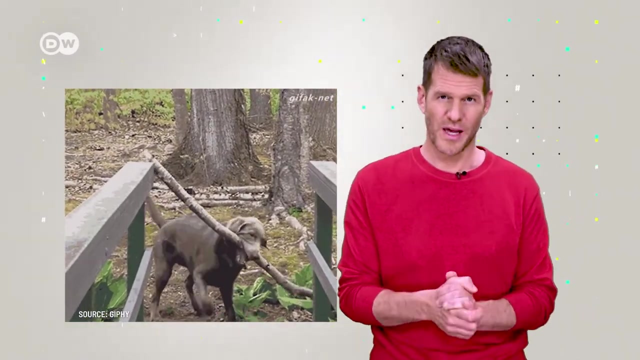 of patients. Beyond being able to score a well-paying job, programming skills also have personal benefits. They help develop creative and cognitive skills. They improve memory and boost brain power, And children, and even us adults, develop problem-solving skills that help relate to the world in general. How Coding essentially involves taking a 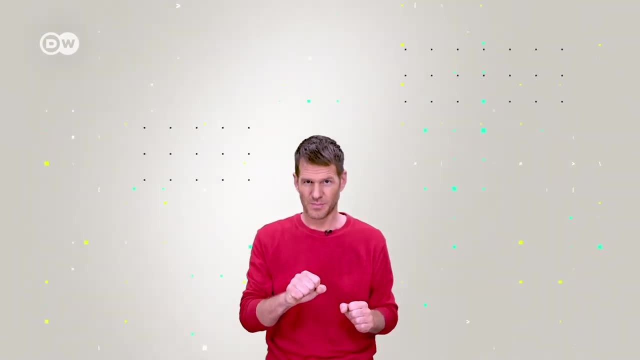 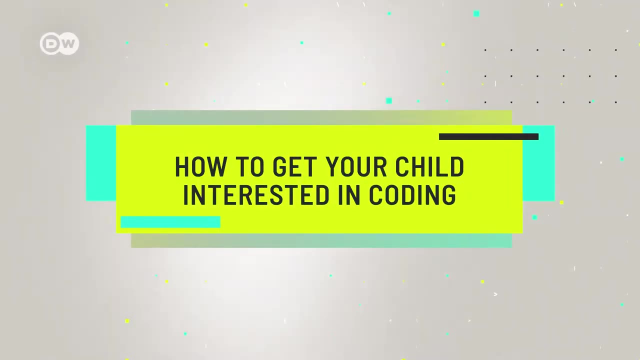 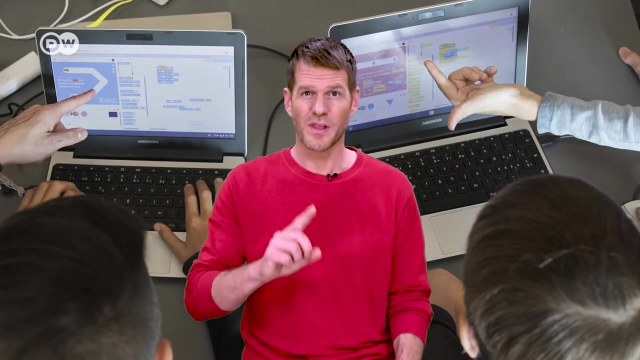 problem and breaking it down into smaller and simpler problems. Once they get used to it, children can approach problems in every other domain of their life in a similar fashion. But how do you get your kids interested in coding? First, find out what they want to create. 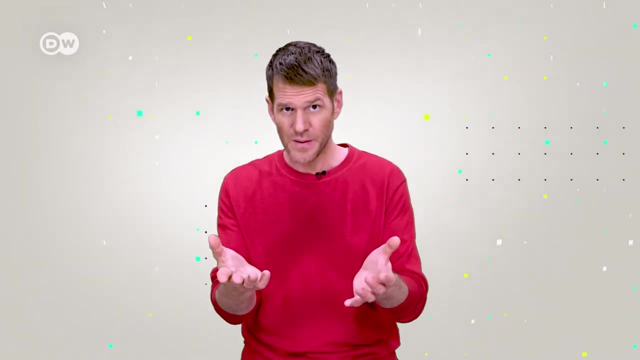 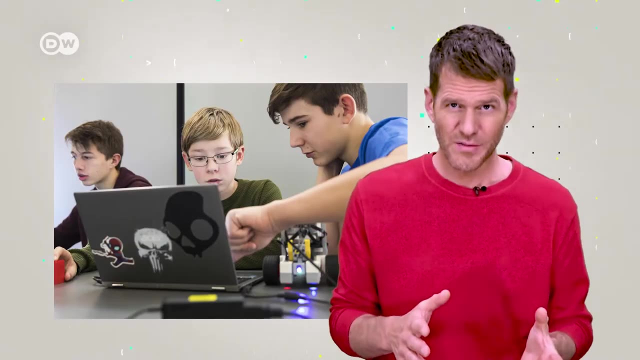 A video game, a robot or an interactive story. And it's even more important to follow their lead, even if their ideas seem absurd at first. Creativity is a key to success, It's a key to success, And it's a key to success. 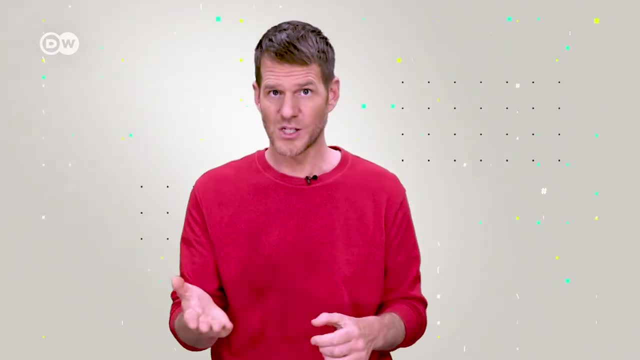 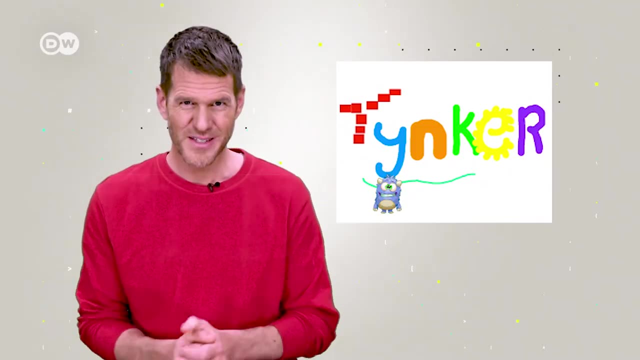 Coding is a kid's main asset when it comes to coding. Programs that teach how to code should thus adapt to that. Here are two examples of programs you can try out with your kid. Tinker is an educational programming platform from the US. It's aimed at teaching children how